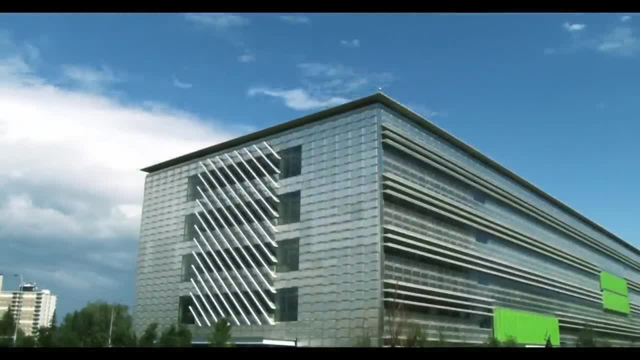 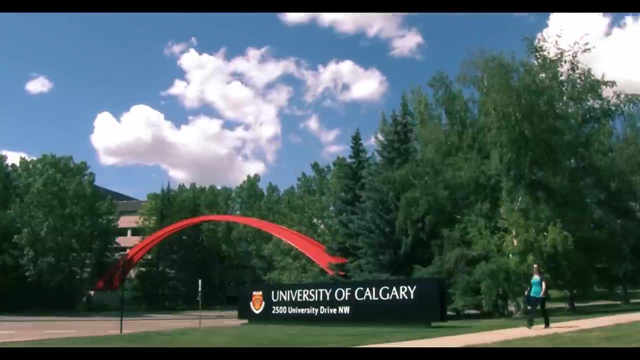 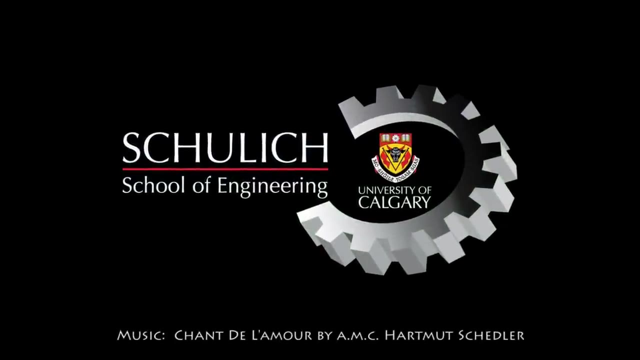 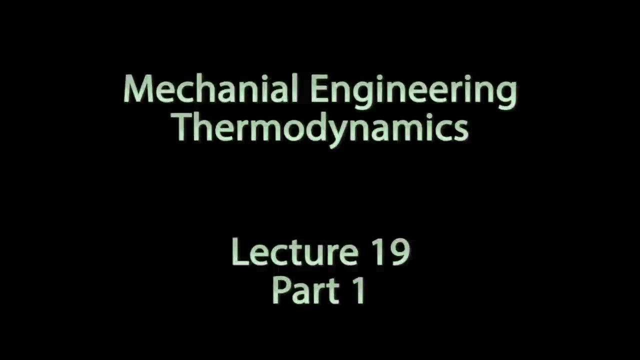 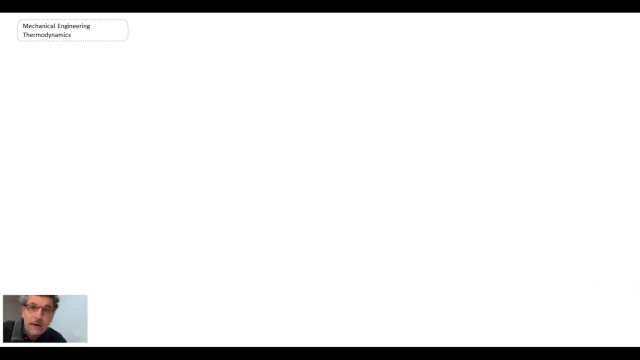 In this lecture. what we're going to be doing is we're going to be taking a look at power cycles that involve vapor, And so we'll have a liquid. the working fluid of our power cycle will be going through a phase change, And one of the 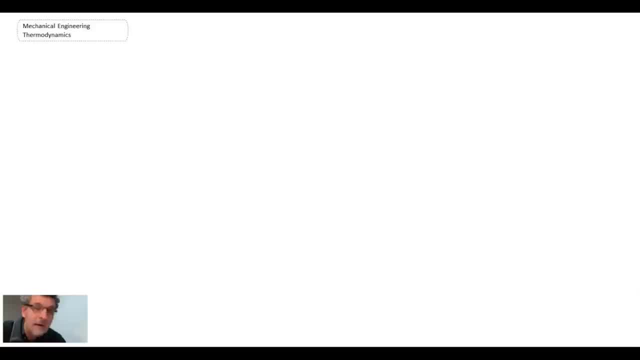 common fluids that we will find in these vapor power cycles is water, Water going through the phase change from liquid water into steam. So we'll be looking at vapor and combined power cycles in this chapter or in this lecture. So thus far what we've looked at in terms of power cycles. we looked at the gas power cycle. 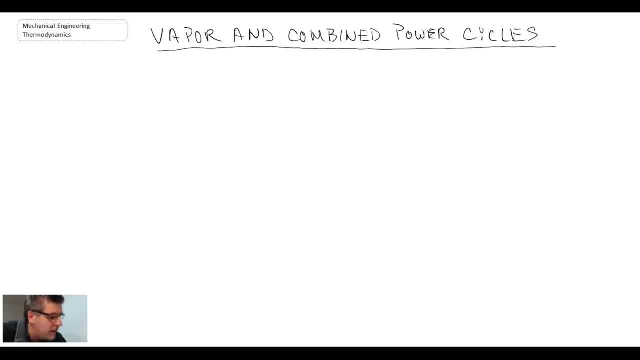 and we considered a number of different ones There. we looked at the auto, the diesel, the sterling and the Brayton. So the thing that we found with the auto, the diesel sterling, perhaps to a lesser extent- and the Brayton, these are gas power cycles that are quite often used in mobile applications. So 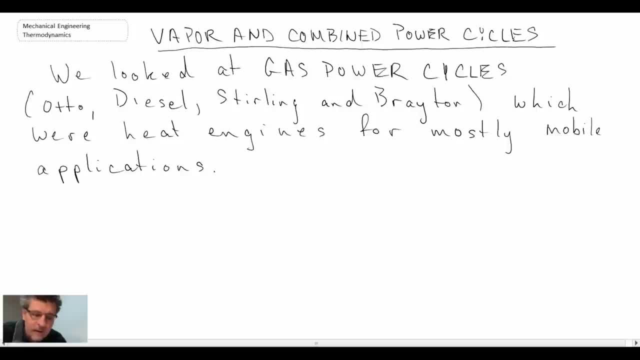 be it an automobile, a ship, aircraft. in the case of a Brayton cycle, We're now going to be looking at vapor power cycles. Now, the thing about vapor power cycles is they have traditionally or historically been used and developed in steam engines. 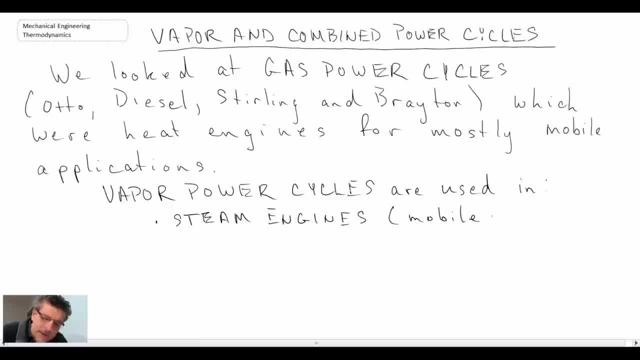 And these were mobile applications. Now, the first one was developed in 1770 by a military engineer for the French army, And then that evolved into steam engines that were used throughout the early 1900s, And in more recent years this has evolved into power plants. So the systems that provide us- 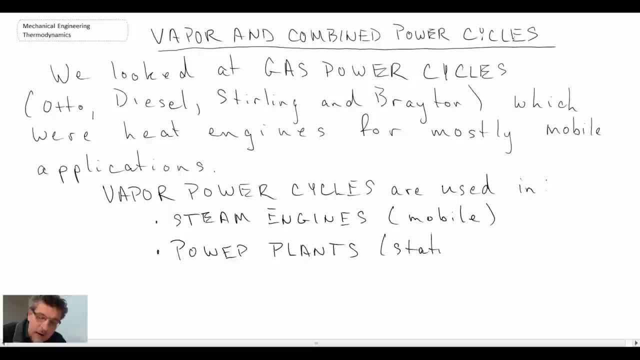 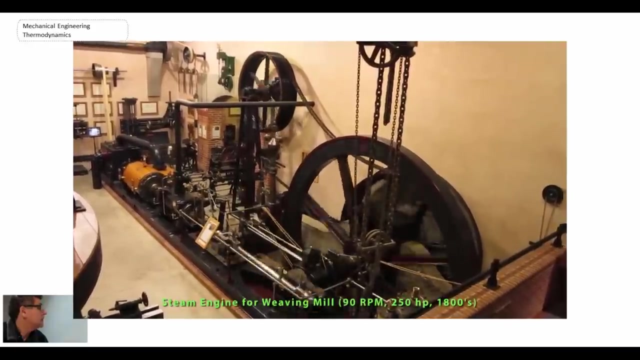 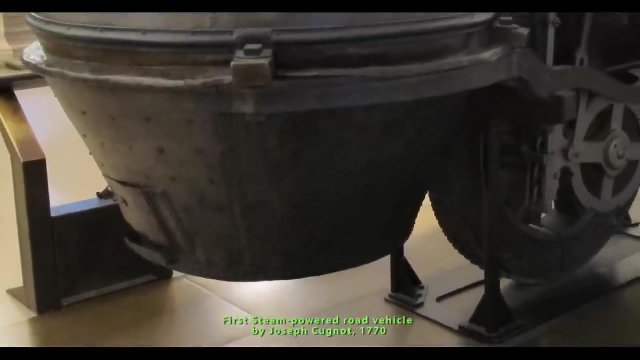 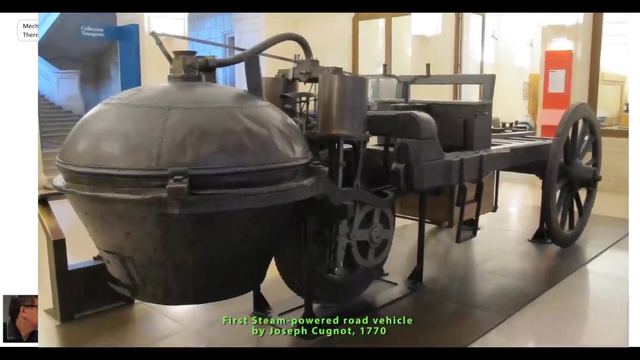 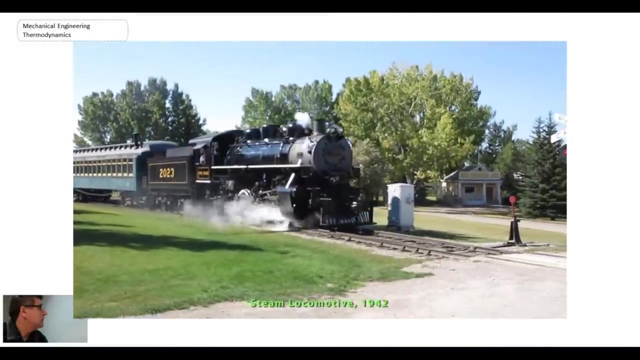 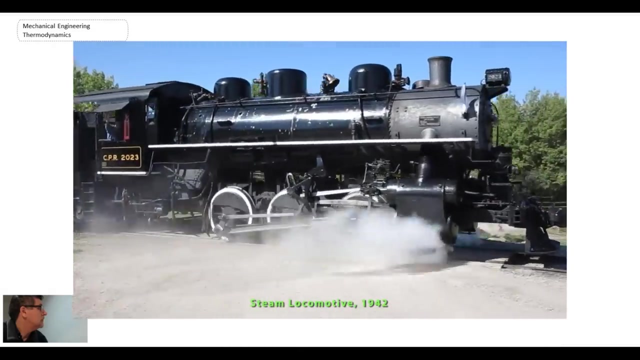 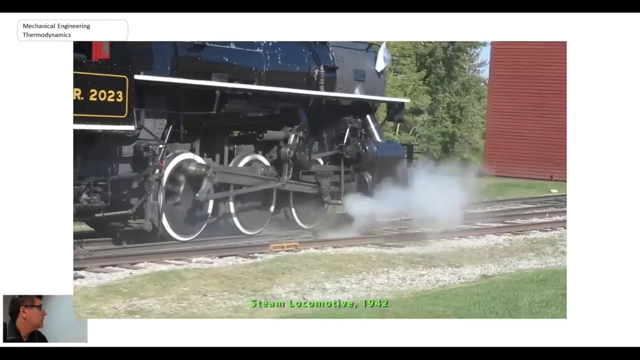 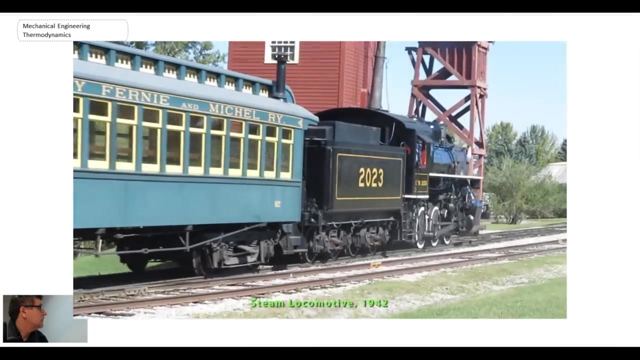 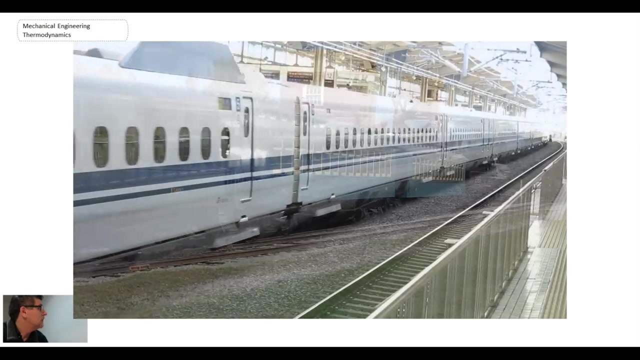 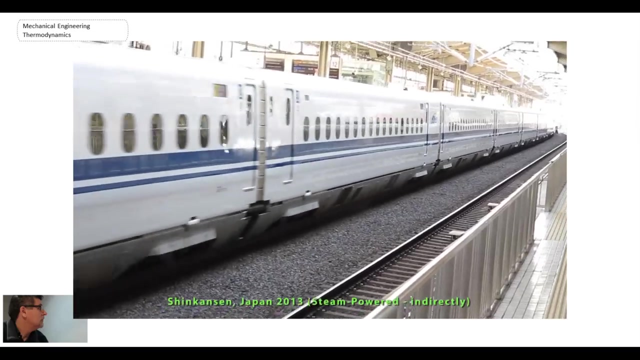 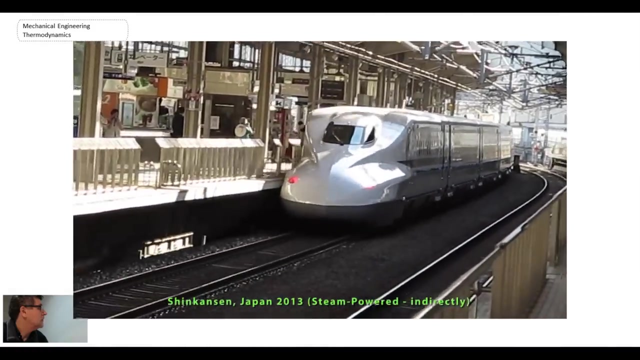 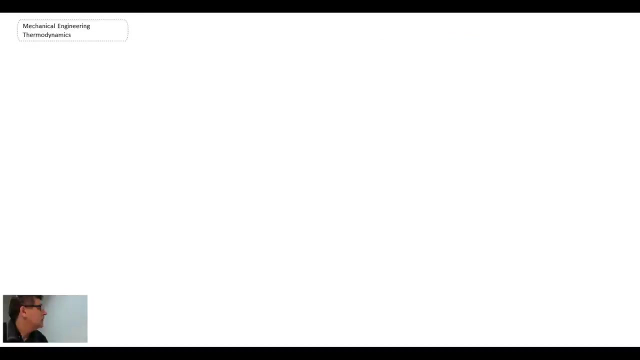 with electricity, and these are stationary. there were also early steam engines that were stationary, as we'll see in the next video clip, so let's take a couple of minutes here and look at a few different applications of steam engines. so so, so in that video clip we saw a number of different applications of vapor power cycles, starting with 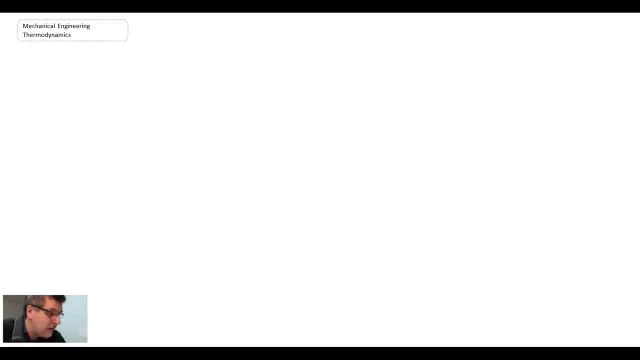 a stationary steam engine that was used as part of a weaving mill back in the late 1800s. we then moved forward. well, actually we moved back in time, but it was the first mobile application from the late 1700s. the french military engineer that i had referred to. 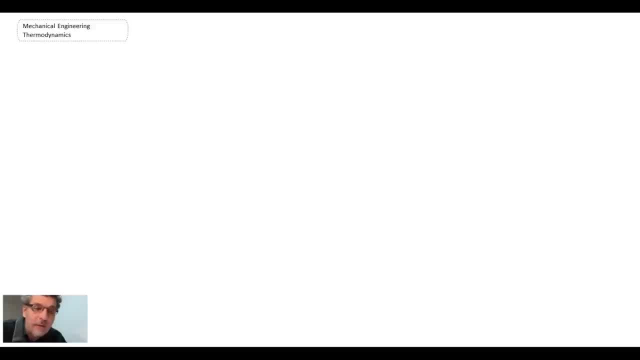 that was the steam engine that was used to move steam from the steam engine to the steam engine- the first mobile application of steam power, where they would build a fire underneath the boiler and and it would generate steam and that system might go for a kilometer or a mile on one single charge. 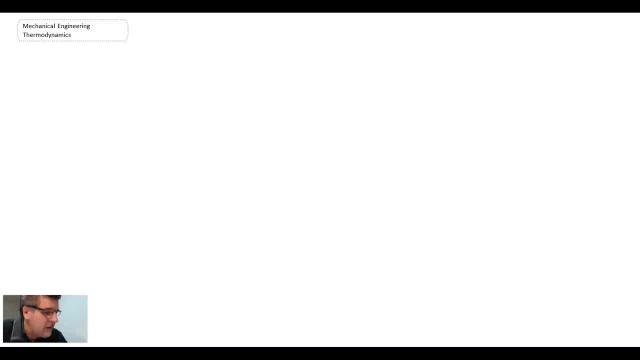 of steam, so it wasn't really that practical. and then then we saw a steam engine that was used in the rail system. that was from about the 1940s era, and and those steam engines were used throughout the world for many, many years and some parts are still used.